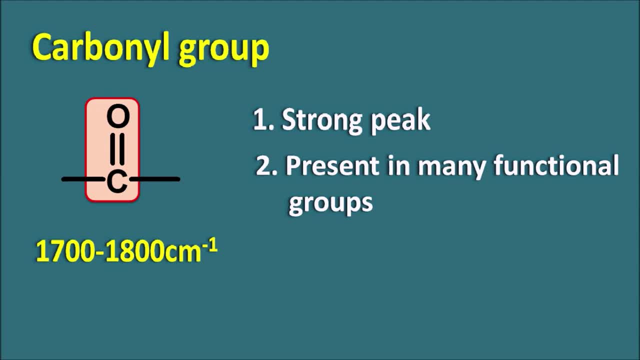 many carbonyl compounds are there which can give this peak, which is an indicator of that peak in a particular compound. And third one: we can easily differentiate this carbonyl group by presence of the other groups attached with the carbonyl group. For example, this carbonyl group is present in the 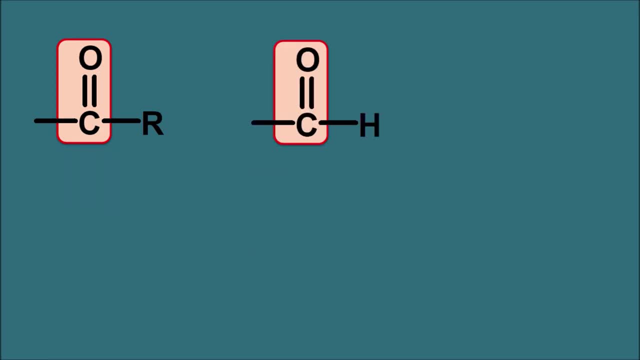 ketones. Otherwise it can be easily identified. So we are going to study the carbonyl group. This group is present in the aldehydes And this group is also present in the carboxylic acids and their derivatives, like the esters, amides and acid halides, even acid anhydrides. In all this carbonyl. 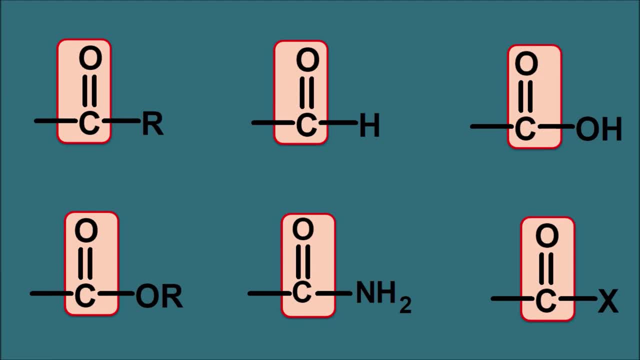 group is present which gives a strong peak in the IR spectra. So if we identify this peak, we can easily identify which type of functional group is present in the molecule. Thereby we can interpret the IR spectra very easily and we can identify the structural features of the. 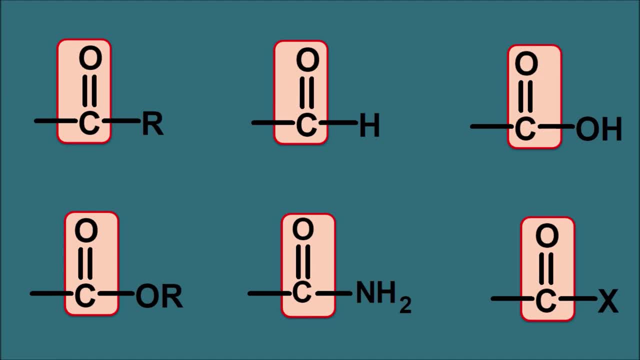 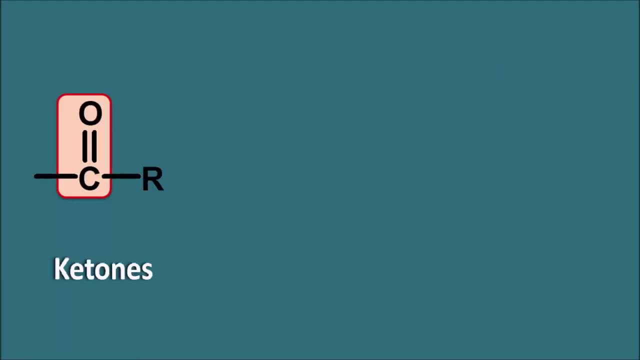 carbonyl group. So this group is also present in the carboxylic acids and their derivatives, like the carbonyl group. However, how we can differentiate this carbonyl peak in these functional groups, Let us take one by one. First of all, let us take the ketones In our previous video. 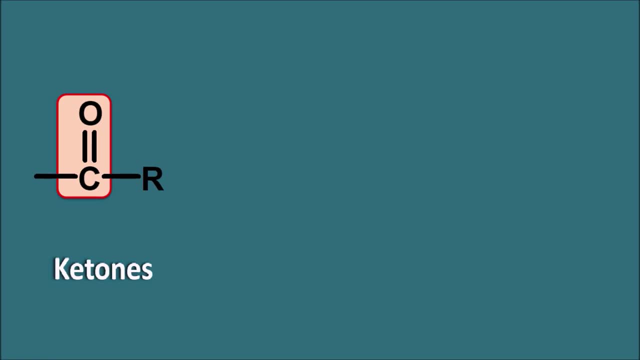 we have already discussed that the IR absorption frequency of the functional group depends on two important factors. One is the inductive effect and second is the resonance. So here this carbonyl group is attached with an alkyl group And this alkyl group produce a positive inductive effect. 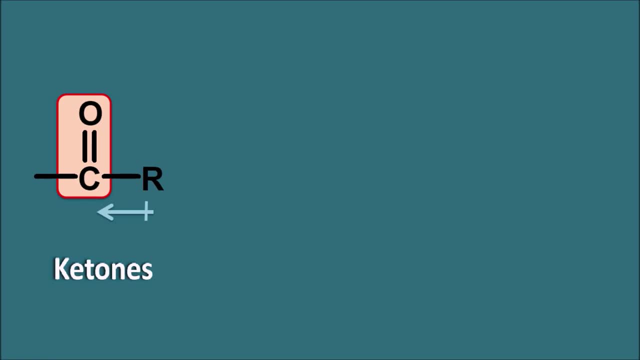 Always the negative inductive effect will increase the IR frequency frequency, but here positive inductive effect will decrease the IR frequency of absorption. Similarly, let us take another function group, that is the aldehydes. In the aldehydes, again, the carmel group is attached with the hydrogen. Here again we can observe the positive inductive effect. 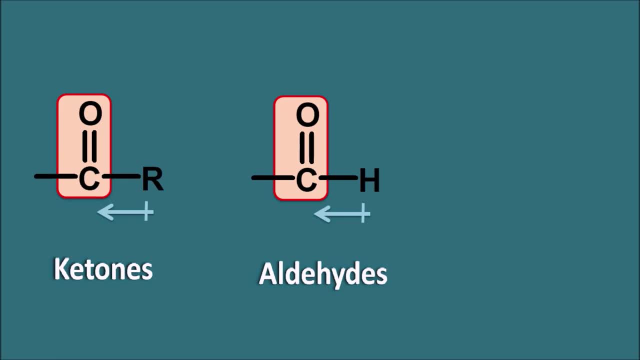 so somewhat less frequency of absorption. and then the carboxylic acids. Now the carboxylic acids are having a carmel group, which is attached with the OH group, because here oxygen is present which shows a negative inductive effect. Thereby the IR frequency of absorption is going to be increased. 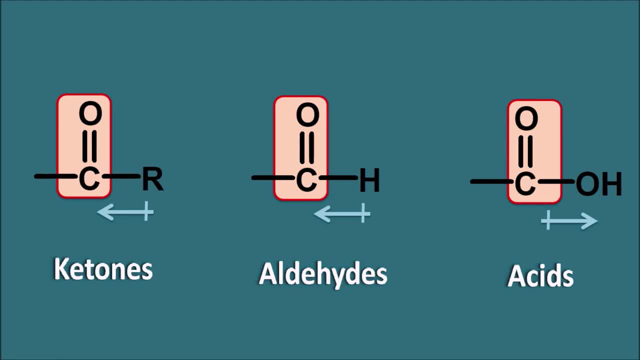 in the carboxylic acids. In this way we can rank these groups, the ketones, as the lowest aldehydes than the acids. We can observe the carmel peak in the ketones at the 17- 10 centimeter inverse aldehyde 17- 20 centimeter inverse and acids at 17- 30 centimeter inverse See. these values are the. 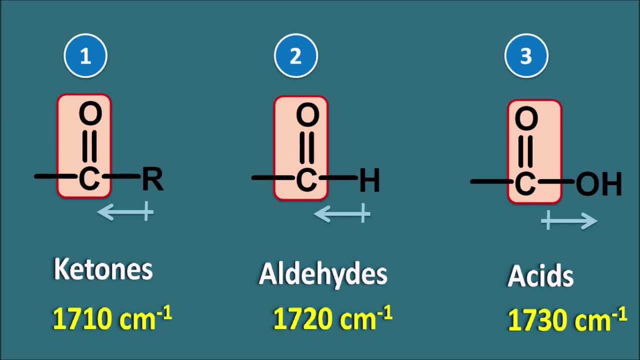 base values. that means we cannot say that ketones are always given negative inductive effect. So when we are giving at the 17- 10, it is variable from 17- 10 to the 17- 25 and by presence of the other groups adsently this value may be slightly changed. So when we are going to remember the IR, 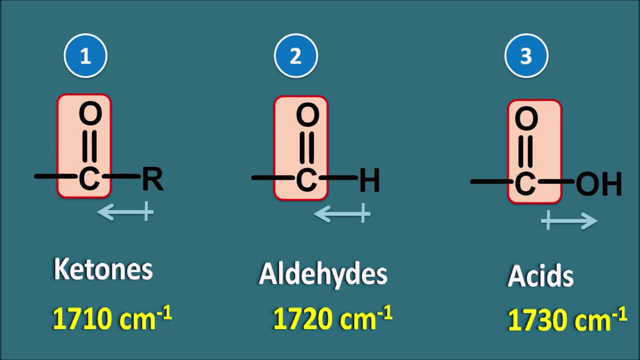 spectral features. you can forget the last two digits. For example, ketone 17, 10 and aldehyde 17- 20, that means they are differing by 10 centimeter inverse, and sometimes ketones can also give the peak at the 17, 20 and 17, 25.. So we cannot say that ketones are always given negative inductive effect. 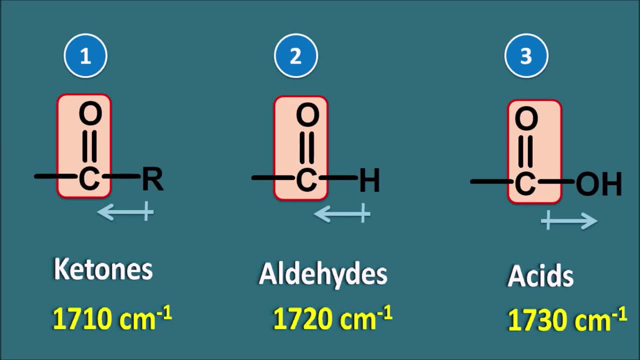 We can now differentiate the ketones and aldehydes by the presence of carmel peak. So these values are the base values in order to remember the position of the carmel peak in the different types of functional groups and we can differentiate these functional groups by the other groups present in. 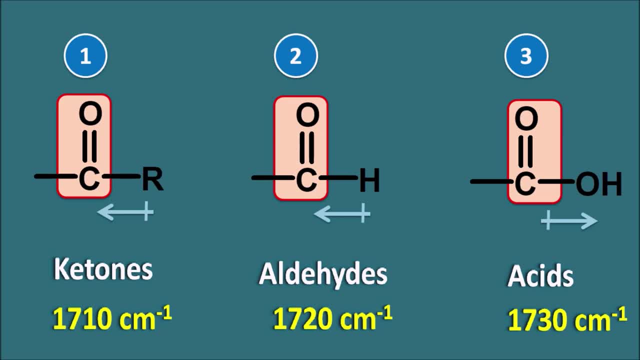 each functional group. So first of all here let us see the position of the carmel groups, then we will go how we can differentiate these functional groups. So ketones at 17- 10 and aldehydes at 17- 20 centimeter inverse and acids. 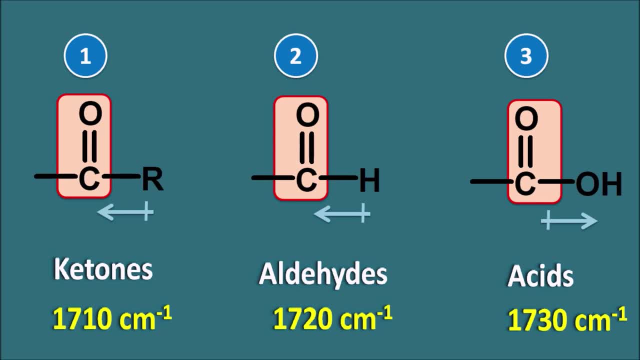 They can show at the 17- 30 as a monomer, but when they are going to form a dimer they can produce a peak at the 17- 10 centimeter inverse. So a lot of variability will be there with the experimental conditions as well as the type of the carboxylic acid and other groups present in the compound. 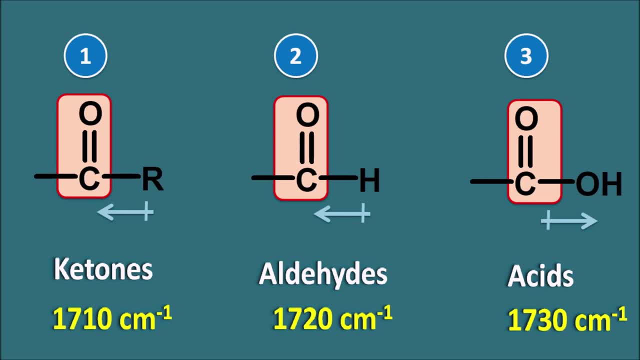 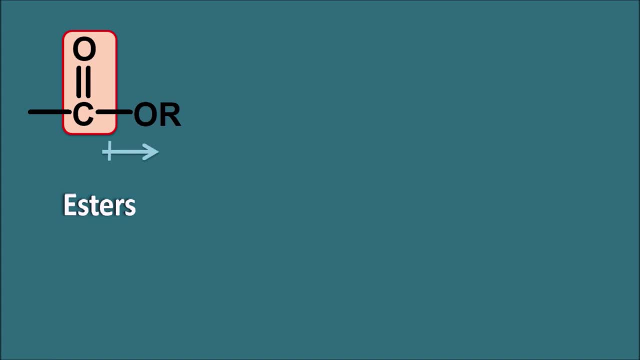 So these are the base values in order to remember the position of the peaks very easily. Then the next one is the esters. Again, in the esters all coccyx group is present, so they show the negative inductive effect. So we can see that the carmel peak at 17, 30 and aldehydes at 17, 20 and 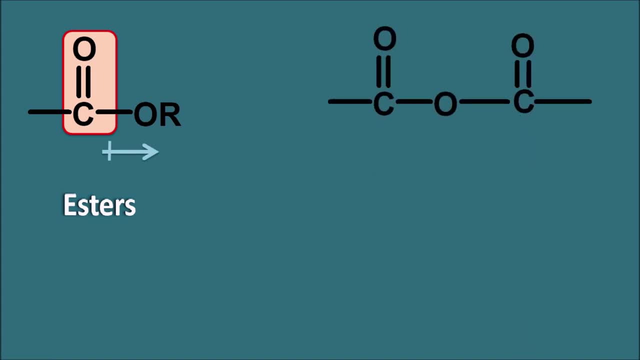 then the acid anhydrides. In the acid anhydrides you can observe two carmel groups are present which are attached with the auxin. So again here the carmel group can show the negative inductive effect. and finally, the acid halides. In the acid halides, halogens are highly electronegative. They show a strong 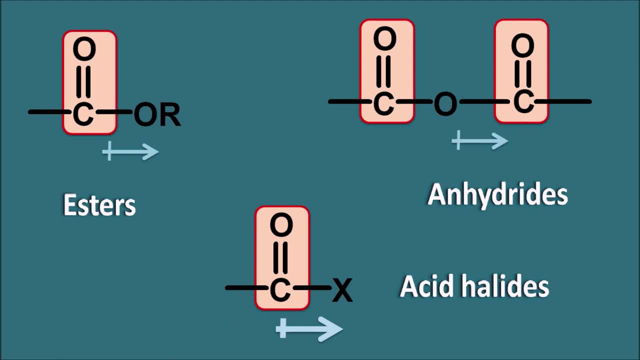 negative inductive effect. So if we continue the ranking, esters can be given the fourth ranking, anhydrides fifth one and acid halides sixth one. Esters will show a strong negative inductive effect. Carmel peak at around 17, 50 centimeter inverse anhydrides 18, 10 centimeter inverse one peak and. 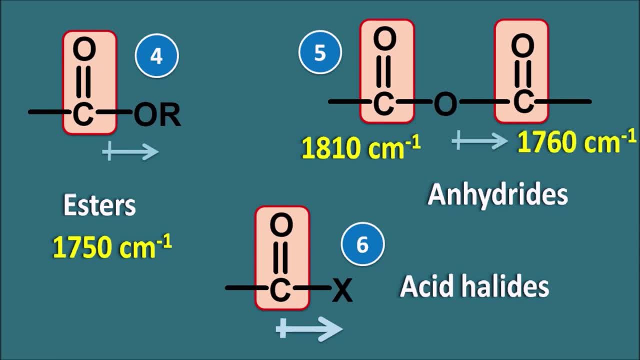 then the another one at the 17- 60 centimeter inverse because it's having the two carmel groups and acid halides at the 1800 centimeter inverse. You can observe in the acid halides we can observe a maximum IR frequency of absorption because of the high electronegativity of the halogens. 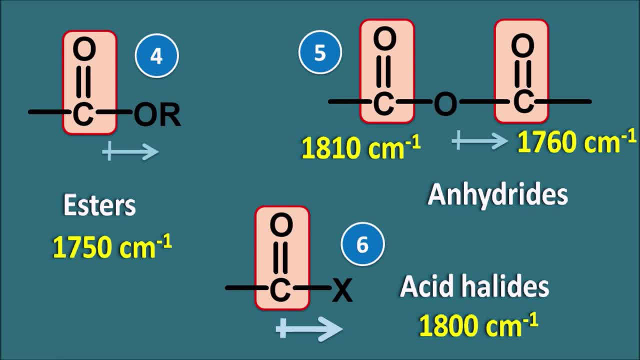 Even anhydrides. we can observe one peak at the 18: 10 because of the electronegativity of the carmel group which is attached at the 18, 50 centimeter inverse. So we can easily differentiate the different types of function groups by studying the other structural 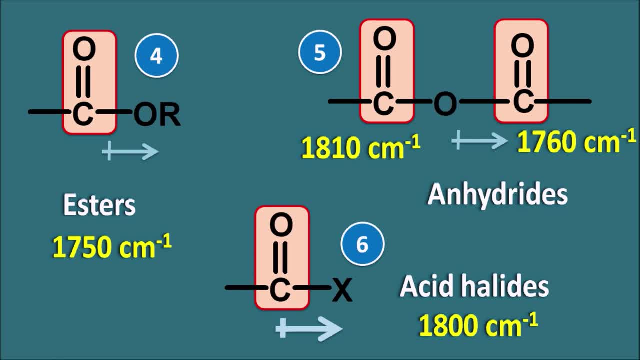 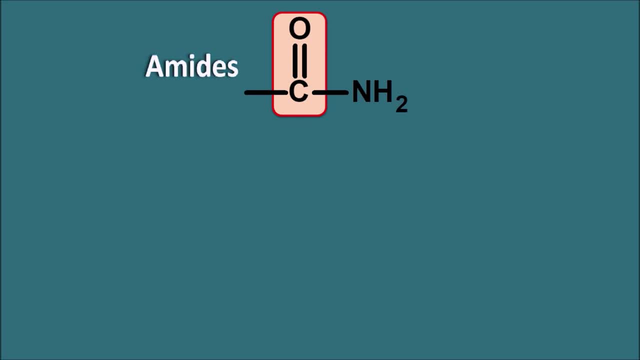 features. But what about the amides? We have not discussed about the amides. Now let us see what happens with the amides. In the amides the carmel group is attached with the NH2 group. So again here nitrogen can show the negative inductive effect. but here not only the inductive effect. 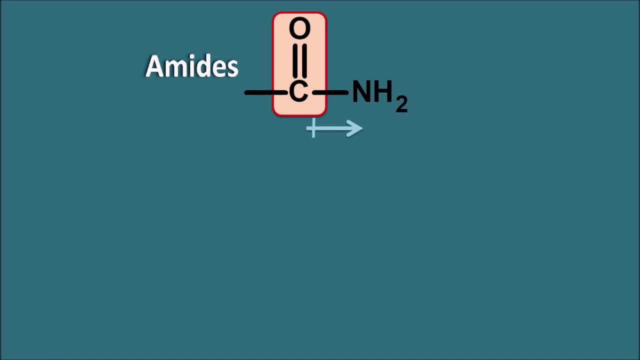 the resonance is also affected by the nitrogen. So here we can see that the nitrogen is attached to the carmel group, which is also going to play its role, For example in the amides. the nitrogen is having the lone pair of electrons which can be easily donated, so it can be donated to the carmel. 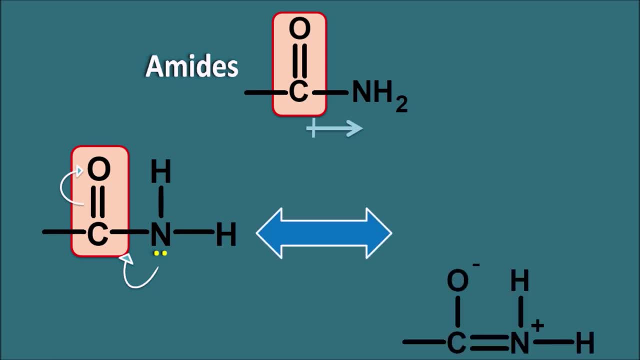 group like this, such that now the amides show a resonating structure like this. In this resonating structure we can observe the carbon oxygen bond is getting a partial single bond character. thereby the bond strength is going to decrease and IR frequency of absorption is going to decrease. 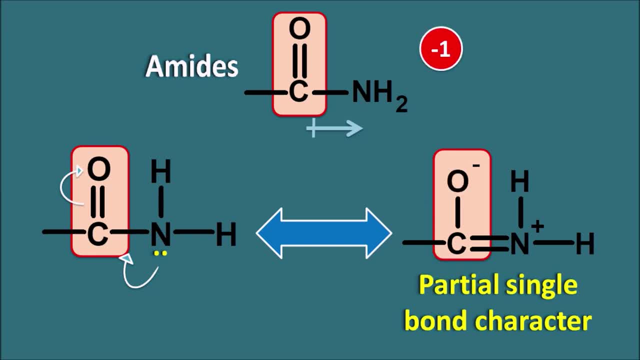 That's why amides will show a low frequency of absorption, so they can be ranked at minus one and they will show at the 1680 centimeter inverse, that means below the 1700.. Now, with this information, let us go with the different types of functional groups and how we can differentiate the 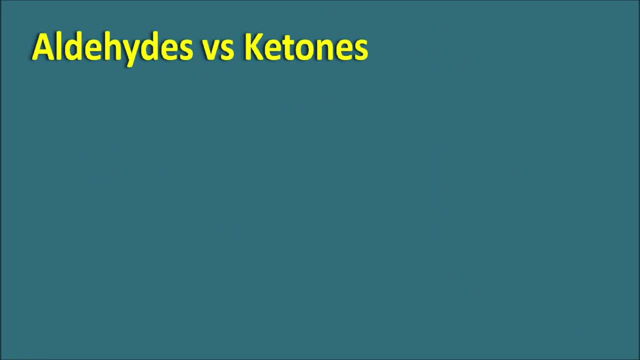 different types of functional groups. First one is the aldehydes and ketones. So this is a structure of aldehydes. Which type of peaks can be observed in the aldehydes? The first one is the carbonyl stretching group, CO stretching. and we can also observe another type of stretching: CH stretching. 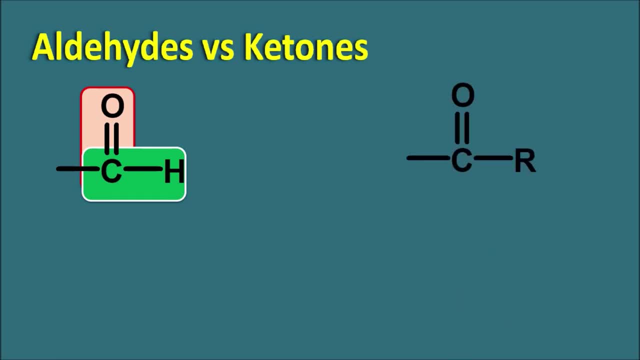 So we can observe two types of peaks here: Ketones. In the ketones we mainly observe the carbonyl stretching peak. So aldehydes will show the two peaks, CO stretching as well as CH stretching. CO stretching is observed at the 1720. 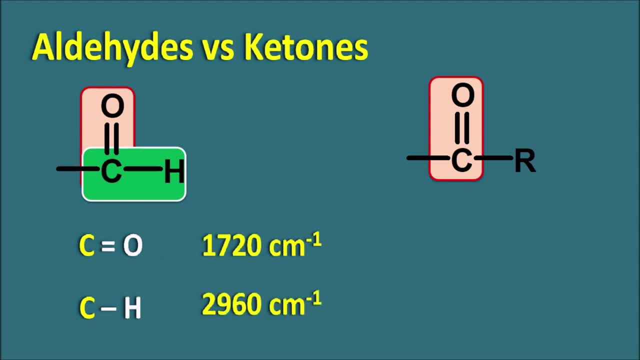 centimeter inverse, whereas CH stretching is observed at the 2960 centimeter inverse. We can simply remember 17 and 29.. On the other hand, ketones will show carbonyl stretching at 1710 to 1720 centimeter inverse, which is variable, but they will not show CH stretching because the 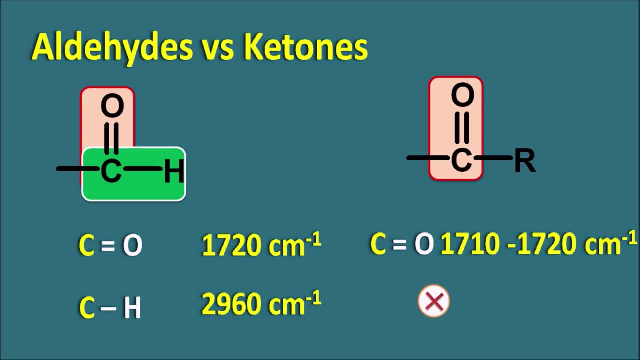 carbonyl group is not attached with the hydrosecond. In this CH stretching the carbon is the carbonyl carbon, not the normal carbon. So in the ketones the carbonyl CH group is not present, so it they cannot show the CH stretching peak, which can be. 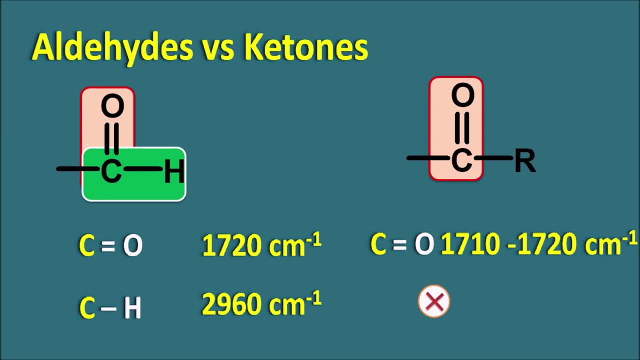 utilized to differentiate the aldehydes and ketones. So in case of aldehydes, we can observe two important peaks at the 1720 centimeter inverse and 2960 centimeter inverse. but in the ketones, we can observe mainly one peak at the 1720 centimeter inverse. 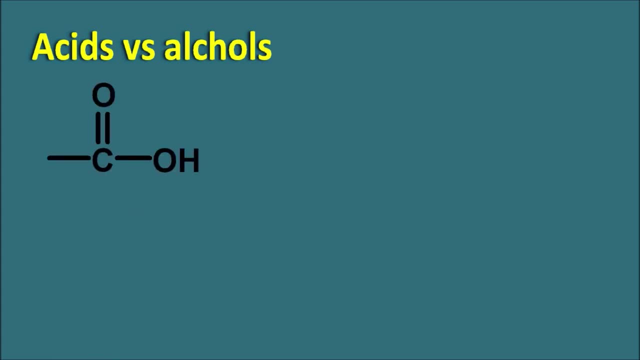 Second one is acids and alcohols. So again in, this is the structure of the acids. here we can observe the carbonyl group. but in the alcohols we cannot observe the carbonyl group and we can observe the alcohol group. So acids are going to show the OH stretching at the 3600. 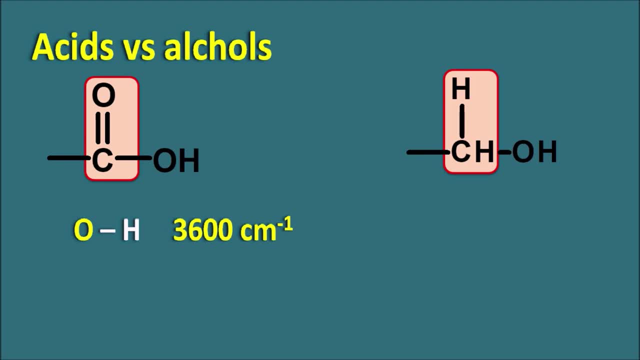 centimeter inverse, which is a free OH group, but when it is hydrogen bonded it show a broad peak. at 3400 to 2300 centimeter inverse. Again, this OH stretching is observed in the alcohols, again at the 3600 centimeter inverse, when it is free and when it is hydrogen bonded we can observe: 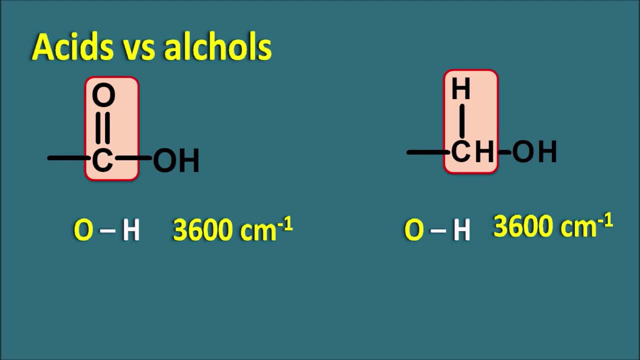 a broad peak, so this feature is not used for differentiation. then second one is the co stretching. co stretching in the acids is observed at the 1200 centimeter inverse, but in the alcohols it is at the 1100 centimeter inverse, say, slight increase in the acids because of the presence of 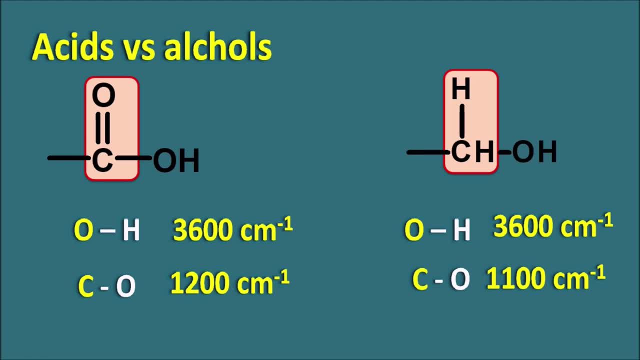 carbonyl group adsently, which increases the frequency of absorption. and then, the third feature is very important: co stretching in the acid is observed at the 17- 30 centimeter inverse, but in the alcohols we cannot observe that type of peak. so alcohols can be differentiated from. 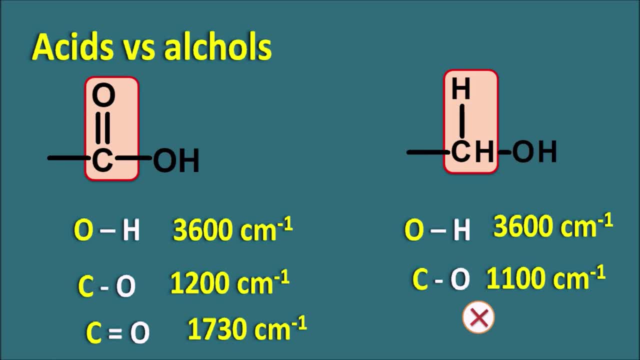 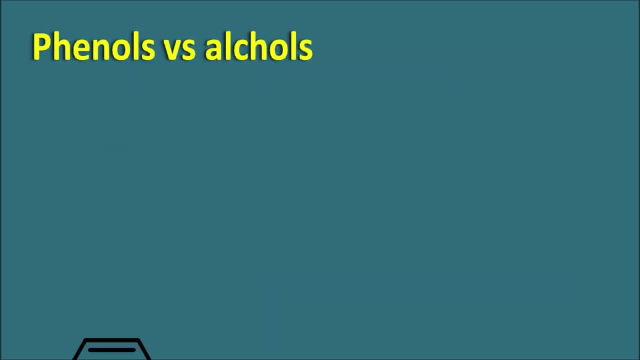 the acids by the carbonyl stretching. carbone stretching is observed only in the acids, but it is not observed in the alcohols. next one is the phenols versus alcohols. so phenols and the oh group which is attached to the aromatic ring system, whereas alcohols and the oh group, which 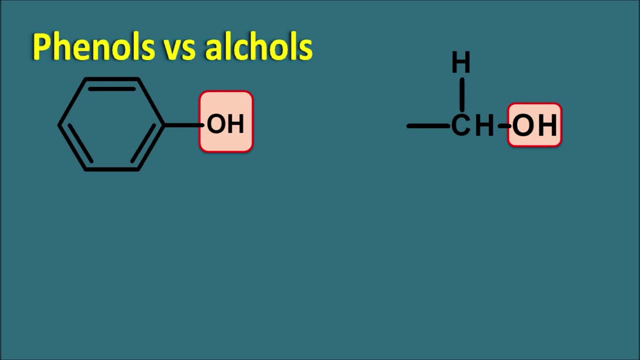 is attached to the alkyl groups. so how can we differentiate these two? in the phenols we can observe the oh stretching at the 3400 centimeter inverse, but in the alcohols we can observe the 3600 centimeter inverse. because of presence of aromatic ring system, the frequency is somewhat decreased to. 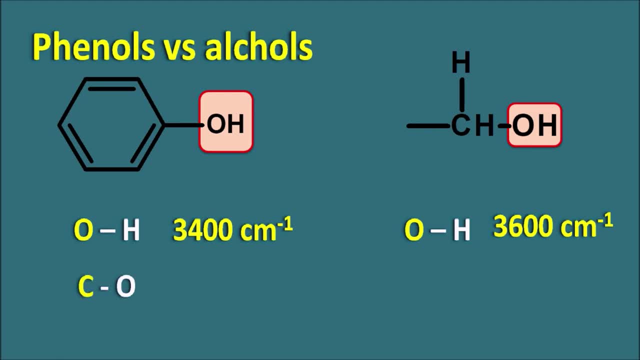 3400 centimeter inverse and co stretching is observed at the 1060 centimeter inverse. again, the co stitching is somewhat reduce compared with the alcohols. in the alcohols it is observed at the 1100 centimeter in verse, a lowering of 40 centimeter inverse is observed in the 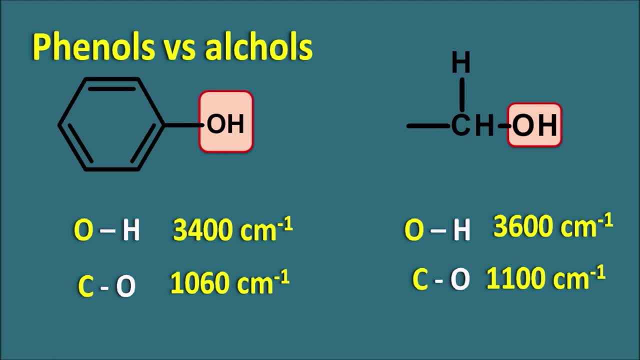 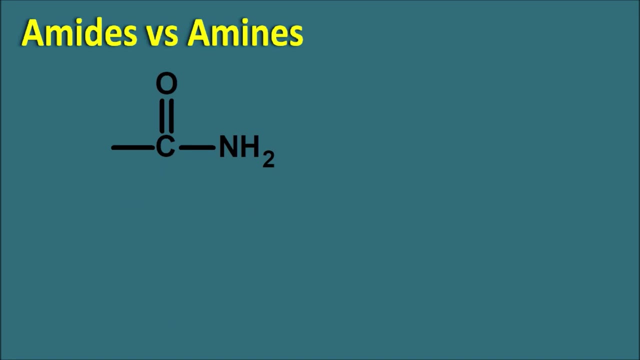 phenols because of presence of aromatic ring system. so in this way phenols and alcohols can be differentiated, where the phenols will show somewhat less frequency of absorption compared with the alcohols. next is the amides versus amines. so this is the structure of the amide, which is: 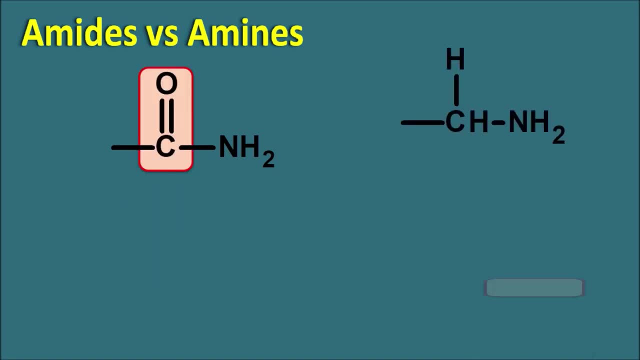 again having the carbonyl function group and this structure of the amines which are having that normal amine group. so in the amides we can observe a nh stretching at the 3350 centimeter inverse. at this position they can show a doublet, which indicates a primary amide, and singlet, which 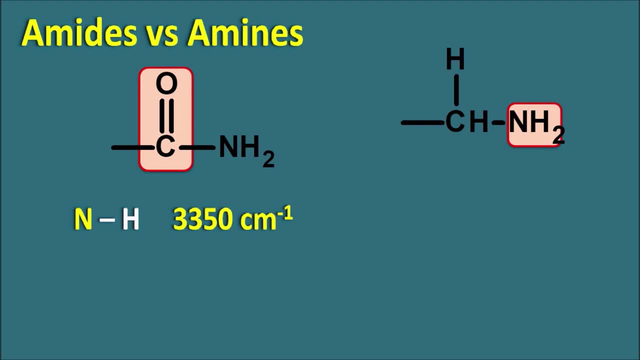 indicates a secondary amide and no peak. it may indicate a tertiary amide. similarly, they can show cn stretching at the 1650 centimeter inverse and in the amines, nh stretching is observed again at the 3350 centimeter inverse, just like the amides. we can observe a doublet if it is a primary amine. 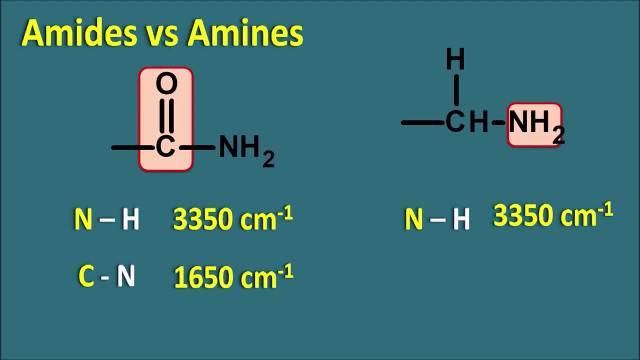 singlet if it is a secondary amine and no peak if it is a tertiary amine. similarly, cn stretching is observed at the 1650 centimeter inverse, just like the amides. but how can we differentiate? the carbonyl function group is present in the amide, which is observed at 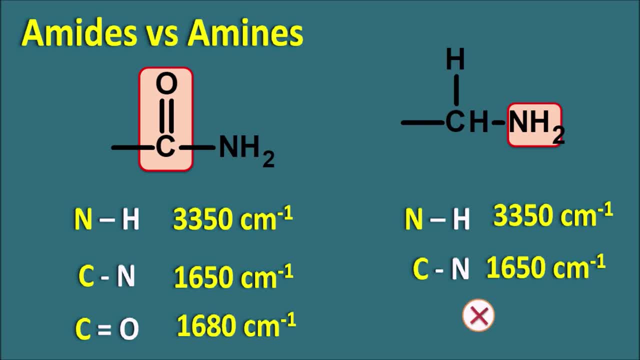 the 1680 centimeter inverse, which is not present in the amines. so this is one point of differentiation. and second thing, the bending vibrations. the nh bending is observed at the 1620 centimeter inverse in the amides, whereas nh bending in the amines is observed at the 800 centimeter inverse. 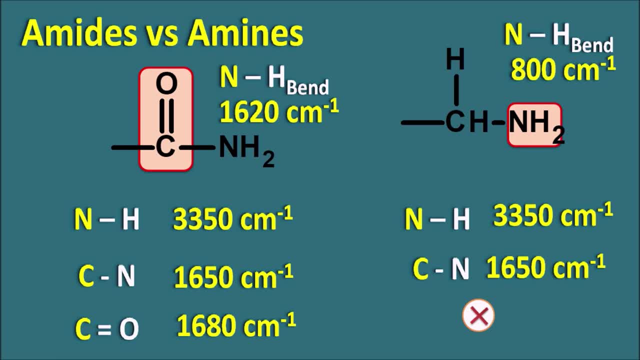 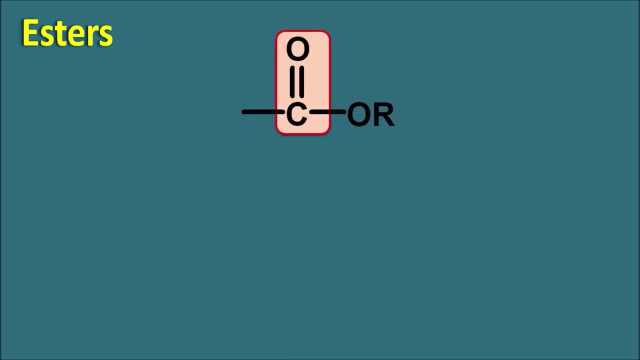 in this way you can differentiate the amides and amines. but the main point of differentiation is the carbonyl functional group. next one is the esters. esters are having function group like this and they can give a co stretching at the 1750 centimeter inverse and co stretching at the 1200. 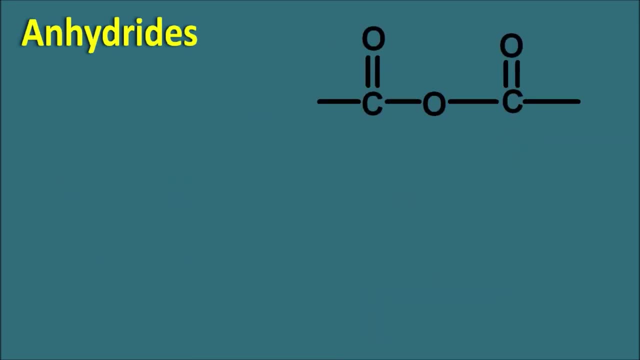 centimeter inverse. next one, anhydrides. anhydrides: already we have discussed they're having the two carbonyl function groups so they can show the carbonyl function groups at the 1760 centimeter inverse as well as 1800 centimeter inverse and co stretching at the 900 to 1300 centimeter inverse. 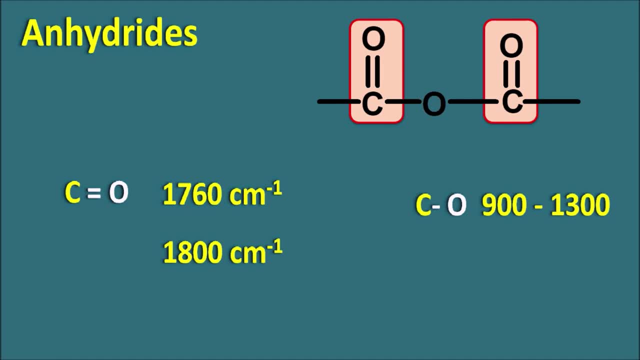 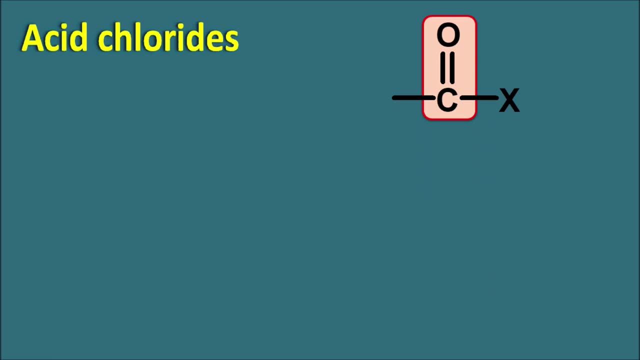 so here co stretching we can observe at the different positions from 900 to 1300 centimeter inverse. next one is the acid chlorides. the acid chlorides, again, we can observe a carbonyl function group along with the halogens. so here co stretching is observed at the 1800. 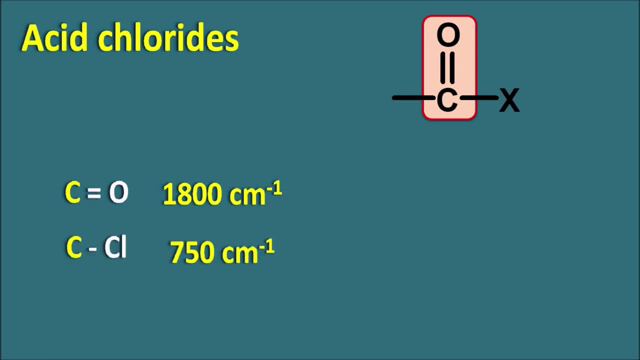 centimeter inverse, and ccl stretching is observed at the 750 centimeter inverse. halides can be differentiated by the presence of the halogen. so, for example, if it is a carbon and fluoride stretching it can be observed at that 1200 centimeter inverse, and carbon and chlorine. 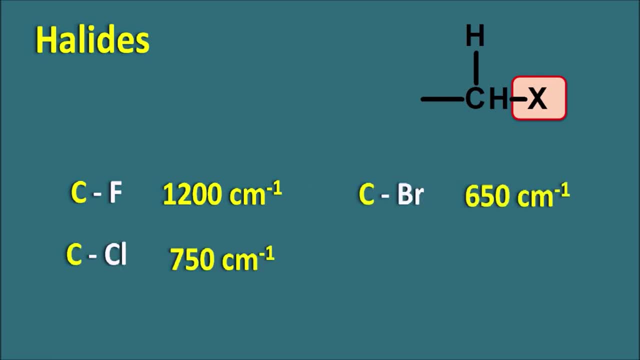 750 centimeter inverse, carbon bromine 650 and carbon iodine 500 centimeter inverse. so these are again the base values by which you can easily remember. as the electronegativity increases, the ir frequency of absorption increases. so fluorine is at the 1200 centimeter inverse halogens are going. 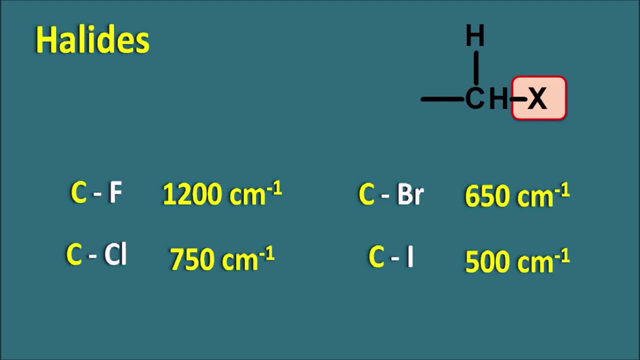 to absorb the hydrogen by the same way. absorption less than 1000. so that's why they can be used as a solvent as well as the material for the making the ir cells, where the halogens are less interfering with our study and bending. vibrations can be observed from 1100 to 1300 centimeter inverse. 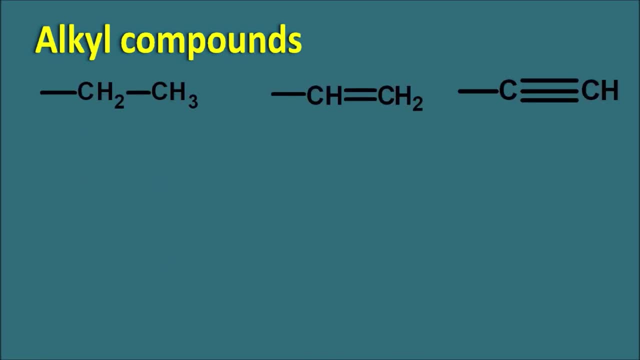 next one is alkyl compounds. we can have alkanes, alkanes and alkynes. in the alkanes, ch stretching is observed at the 3000 centimeter inverse and carbon. carbon stretching is observed at the 1200 inverse and CH bend is observed at the 720 centimeter inverse. In the alkynes, which is a 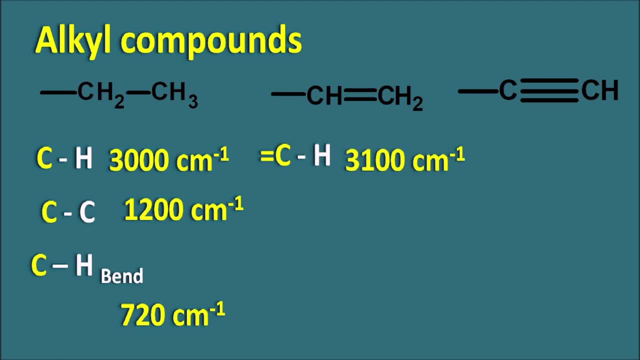 double bond CH. the CH stretching is observed at the 3100 centimeter inverse because the carbon is attached to a double bond and the CC stretching is observed at the 1600 centimeter inverse and the CH bend is going to be observed at the 1000 centimeter inverse. Similarly, alkynes 3300 CH. 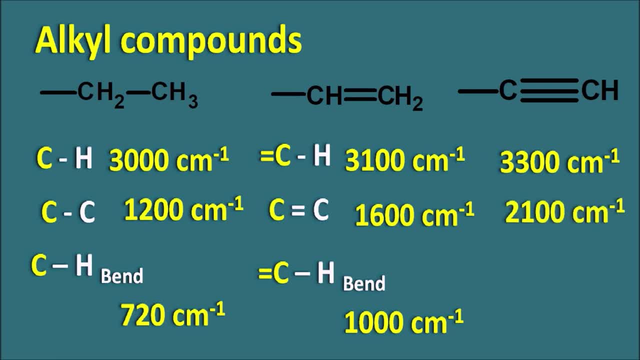 stretching. CC stretching at the 2100 and CH bending is not that much significant in the alkynes. How can we differentiate the alkynes? You can easily remember the CH stretching is respectively 3000, 3100 and 3300.. You can simply remember 30,, 31,, 33.. Similarly, CC stretching 12,. 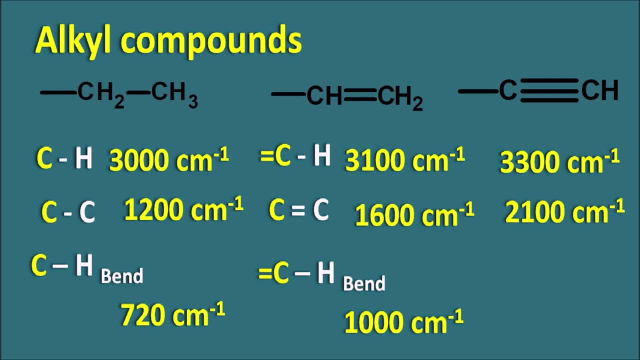 16, 21,, which are different by 4 and 5 respectively. so 12, 16, 1621.. If you just remember these base values, you can easily identify the position of a particular peak in the IR spectrum and particularly the value of IR absorption. frequency cannot be fixed. 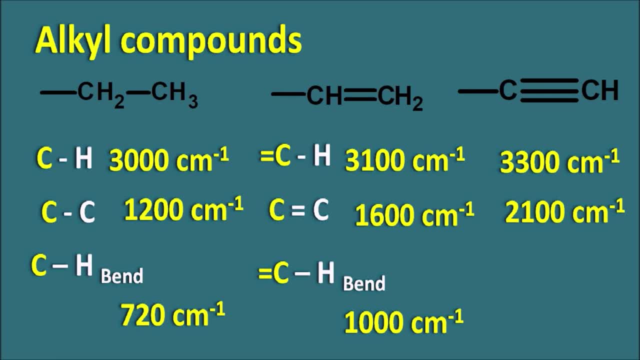 to a single point, because the IR frequency of absorption depends on the experimental conditions, as well as the groups present in the molecule and what are the solvent we are using. So many factors can influence the the exact position of the IR peaks within the IR spectroscopy. So it's 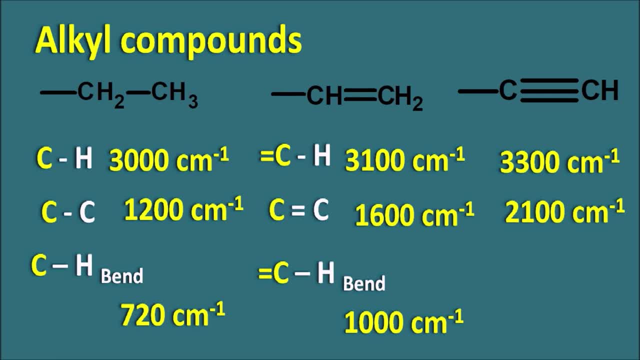 always better to remember the base values in order to identify the relative position of the peaks in the IR spectrum, So this is one of the easiest way to remember and interpret the IR spectra. Hope you have enjoyed this video. If you like this video, please subscribe to our channel. 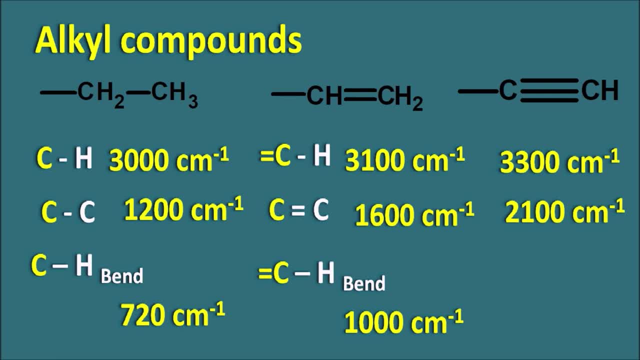 share this video with your friends. post your comments in the comment box. Thank you for watching this video. Thank you for watching this video.